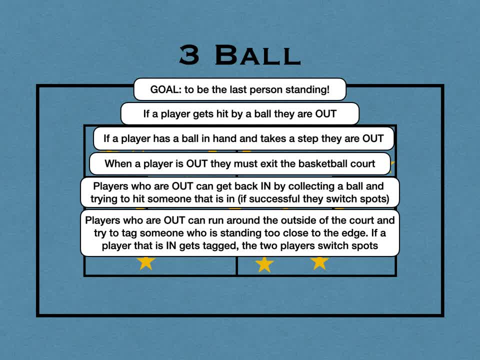 If a player that is in gets tagged, the two players switch spots. So that's two different ways that the players who are out can get themselves back in: If they can hit someone with a ball or if they can tag somebody who's just hanging out and not paying attention too close to the edge. 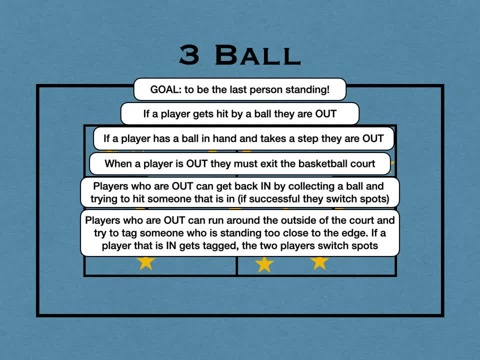 But the players who are out cannot step onto the ball. They step onto the court to do that, And the last rule here is if a player that is in steps out, then they're out. So you've got to watch where you're going. 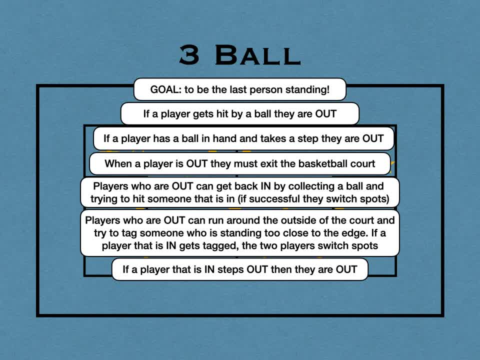 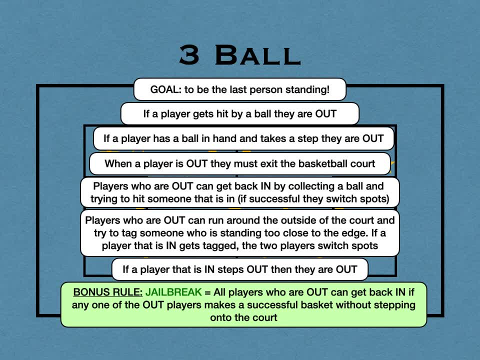 If you're inside the court and you accidentally step on the line or out, then you've got to go out And there's an extension here that you can use if you want. You don't have to, but it's a bonus rule, a jailbreak rule, that all players who are out can get back in if any one of the out players makes a successful basket without stepping onto the court. 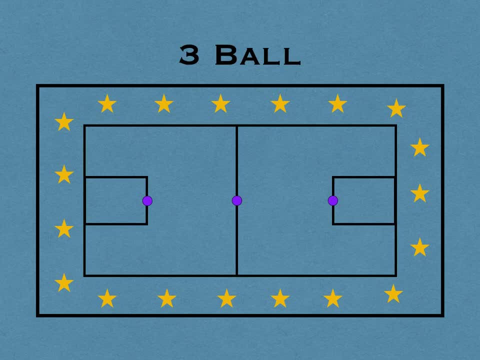 And we'll look at that rule in a little bit here. So again, we're going to start from the beginning. There's a ball outside, Teacher blows the whistle, Players enter the court And some get to the ball, Some don't. 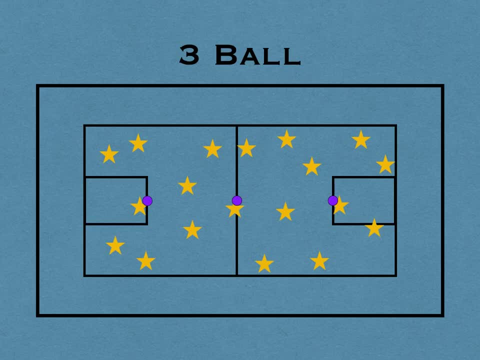 Now you have to imagine that the players that don't have the ball, they're going to be always moving around. So I don't have it on the animation here, but everyone's moving around trying to dodge the balls and so on. The players that have a ball cannot move. 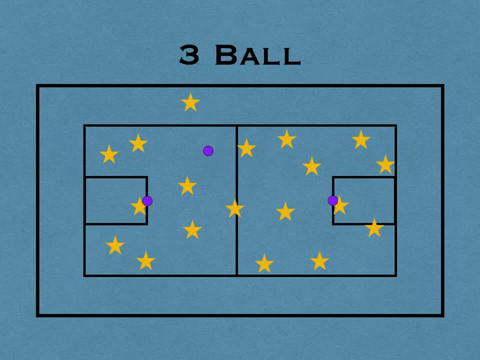 And so if a player throws it and somebody gets hit, that player has to leave the court, They're out, And meanwhile a player is walking with a ball Not allowed. Oh, they realize. Or somebody says, hey, you're walking. 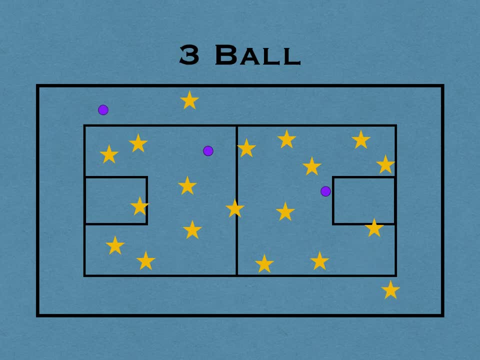 Then they've got to jump out. They're also out And the player is thrown, Missed. And now the player that's on the outside- they've gotten that ball And remember players on the outside. if they throw a ball and hit somebody, then that player is out. 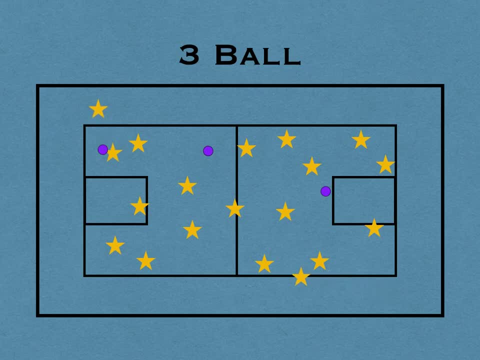 And they've saved themselves and they're back in And we see one player has snuck up on somebody and tagged the player who wasn't paying attention. So that player is out And they have saved themselves as well, And the most common way that people are out is, of course, just getting hit by a ball. 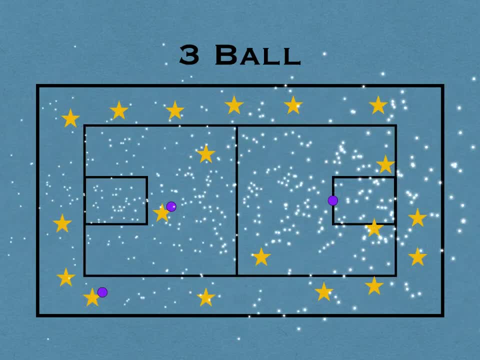 And then they've got to jump out. So what we're going to do is we're going to imagine the game has gone on for a while And a whole bunch of players are out, And if you remember that bonus rule, So again the jailbreak rule. 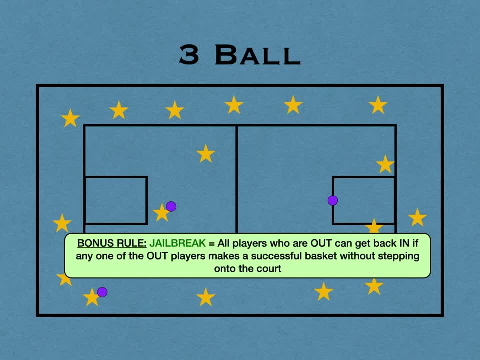 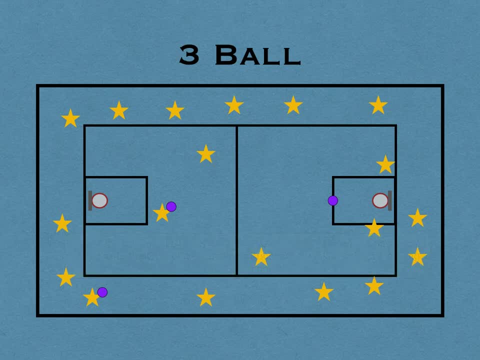 Everyone who's out can get back in if somebody who's out makes a hoop. So obviously we have the hoops in here And this is a good time to talk about the players who are out. If they have a ball on the outside, they can walk with it.